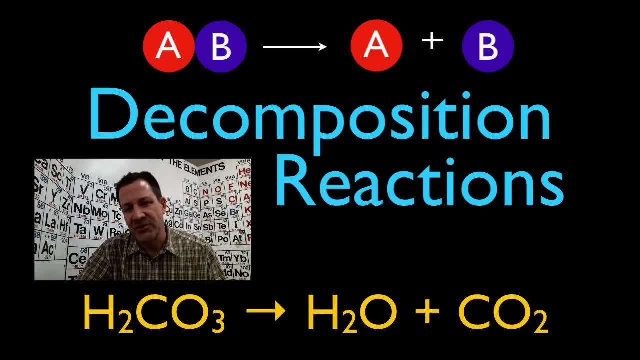 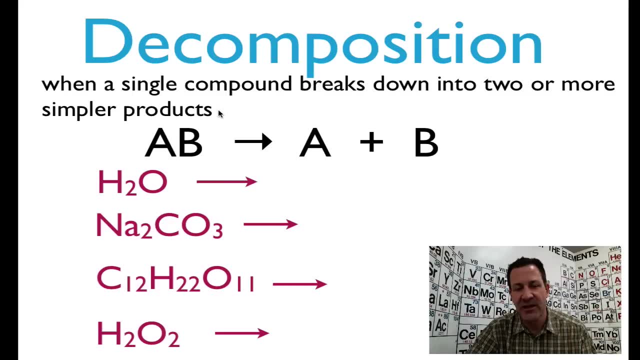 Okay, in today's video I'm going to be going over decomposition reactions, And decomposition reactions is when a single compound breaks down into two or more simpler products, And you can identify decomposition reaction by the fact that you have a single compound on the left-hand side. 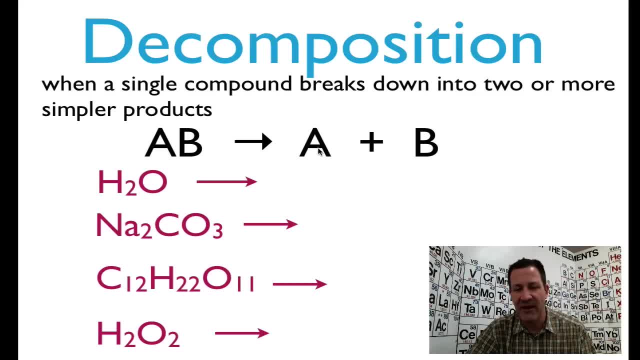 on the reacting side of your chemical equation And the right-hand side, you're going to have that compound broken down into simpler components. So these are the products A plus B and this is our compound on the left-hand side. You see, we have a single compound on the left-hand side of our chemical equation. 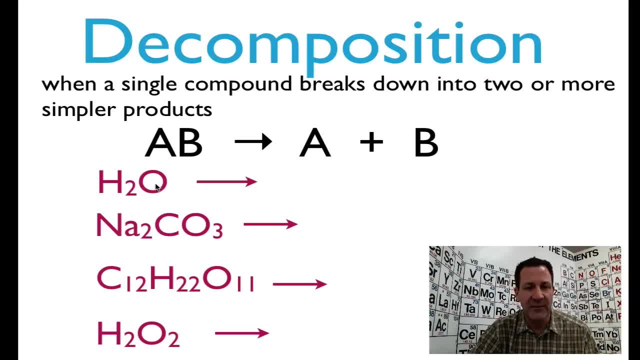 All right. so here we have some decomposition reactions that we're going to do or some compounds that we're going to decompose, And let's go through and let's see if we can figure out what the products are going to be and then also balance those chemical equations. 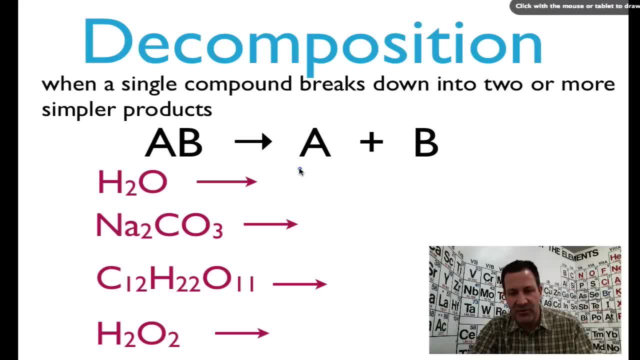 So we have water, H2O. We're going to decompose that. That's commonly done by electrolysis. So we know we're going to have hydrogen and oxygen. Those are our two elements And it's going to be broken down into elements. 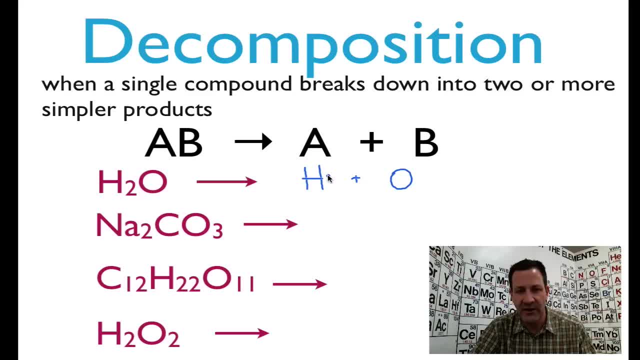 So we want to know: is it just hydrogen and oxygen like that H2O, Or is it something else? So we want to remember we have our diatomic gases, And you can remember the diatomic gases using this term: Brinkelhof. 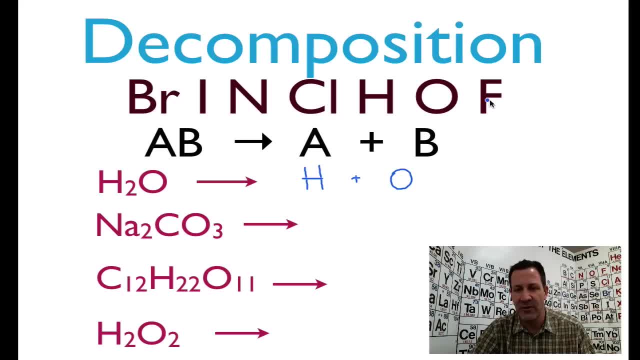 We have bromine, iodine, nitrogen, chlorine, hydrogen and oxygen and fluorine. Those are the diatomic gases. So you can see we're going to have H2 plus O2, oxygen gas and hydrogen gas. They don't exist as elemental hydrogen and elemental oxygen. 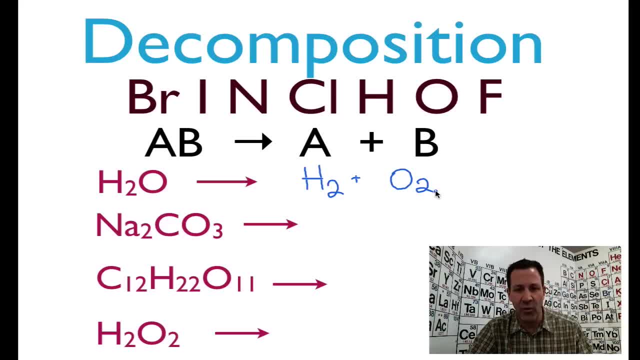 All right. so that's the decomposition reaction for water into hydrogen and oxygen. We know we have our diatomic gases And, let's see, we want to balance this. We have two hydrogens and two oxygens, So we're going to put a two here. 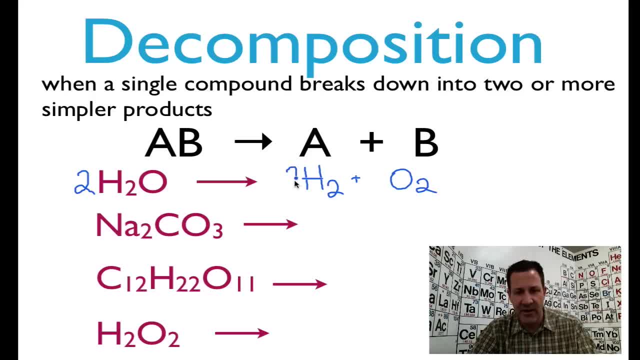 That gives us four hydrogens, And that means we're going to have to put a two here, And I think that chemical equation is balanced just like that. Okay, now we have sodium carbonate, And sodium carbonate is going to decompose into two other compounds. 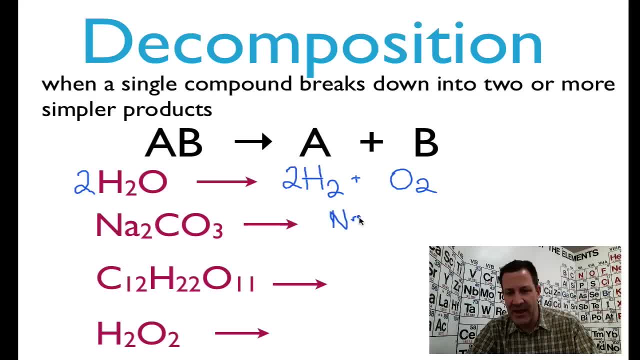 All right and we're going to have NaO, sodium oxide, But we know that oxygen is minus two and sodium is plus one, So we're going to have to put a two right there for our subscript. So that is at the neutral charge overall. 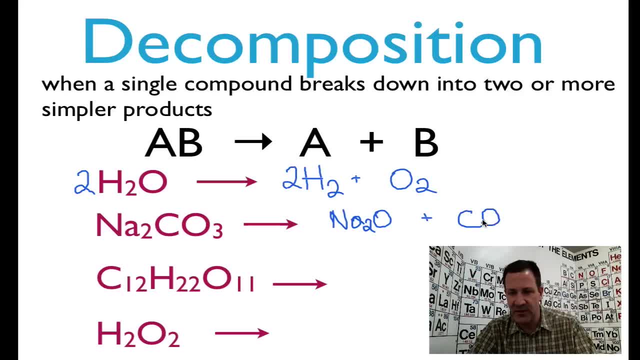 And then we're going to also have carbon dioxide, CO2.. And I believe, two sodiums, one carbon, three oxygens. I believe that is balanced just like that. Okay, now we're going to decompose sugar, And we can decompose sugar using a strong acid like sulfuric acid as a catalyst. 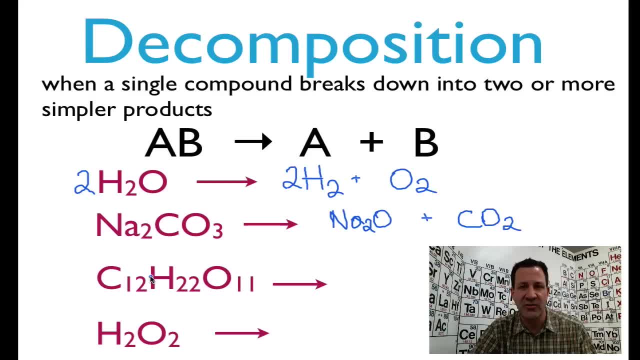 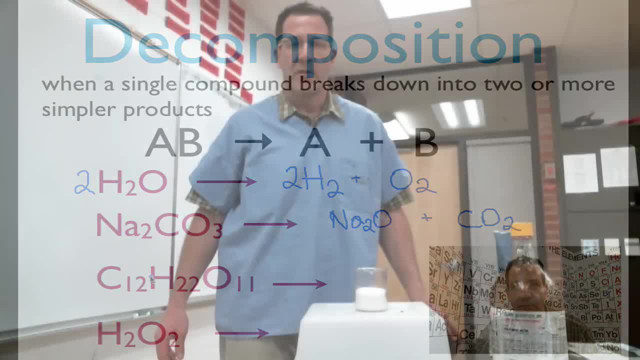 So let's go through- and I'm going to show you that Decomposition reaction before we go through- and predict the products and balance that equation. So let's go do that right now. Okay, we're going to do decomposition of sugar. This is just plain sugar I bought at the store. 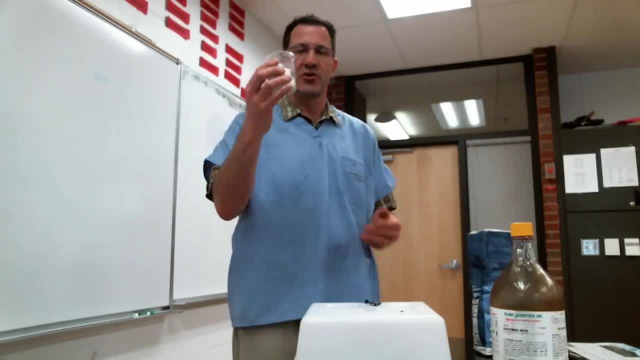 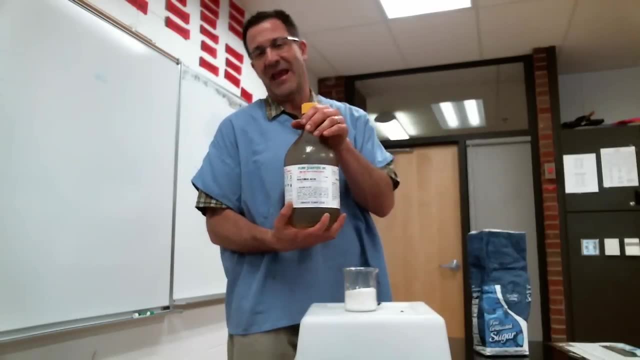 I have about plain granulated sugar. I have about 100 milliliters of sugar in my beaker, And then to that, as my catalyst, I'm going to add concentrated sulfuric acid. This is 18 molar sulfuric acid. 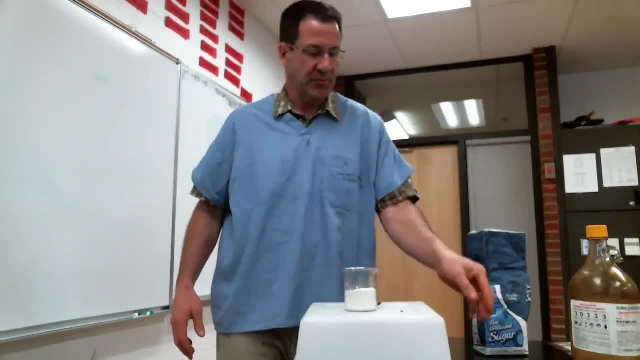 I'm going to be very careful. It's very nasty. So I have about 100 milliliters. I have about 100 milliliters of sugar. I have about 50 milliliters of concentrated sulfuric acid. I'm going to add the two. 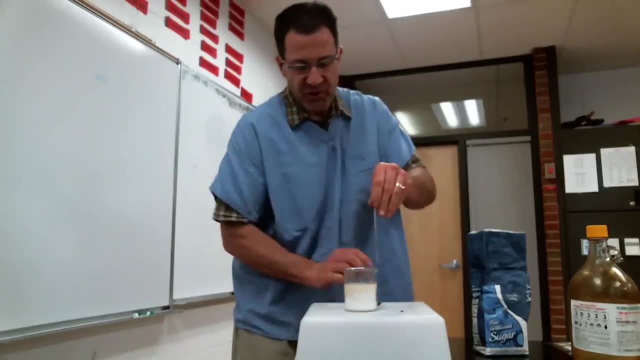 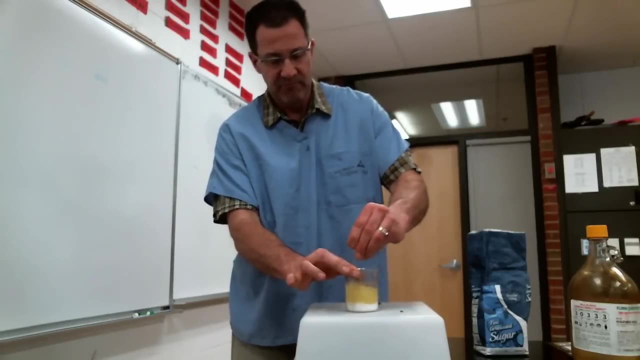 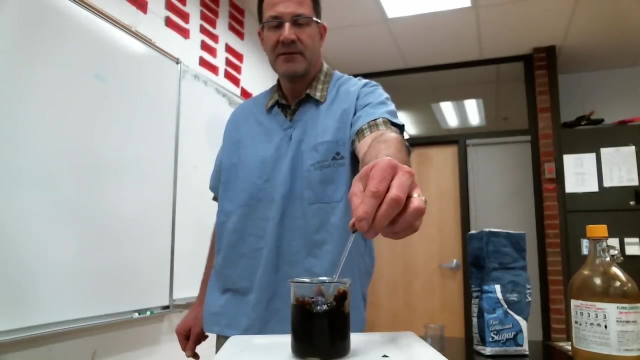 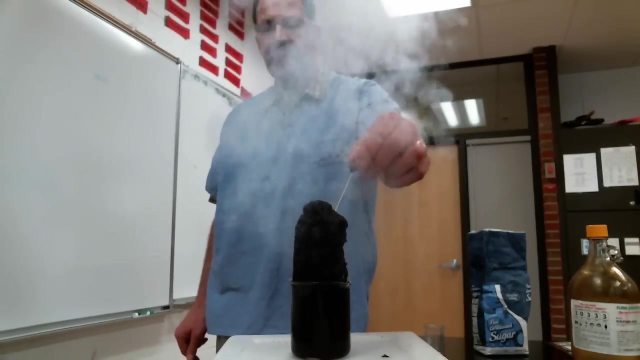 And I'm going to stir it. You'll see pretty quickly it's going to start to change color. Get it all mixed up nicely and starting to react. You can see It's decompositing the sugar. That's decomposition of sugar. 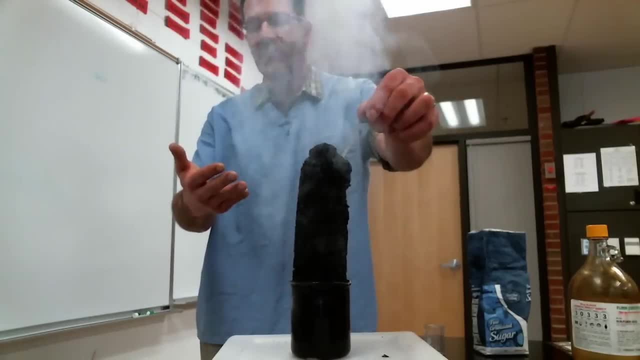 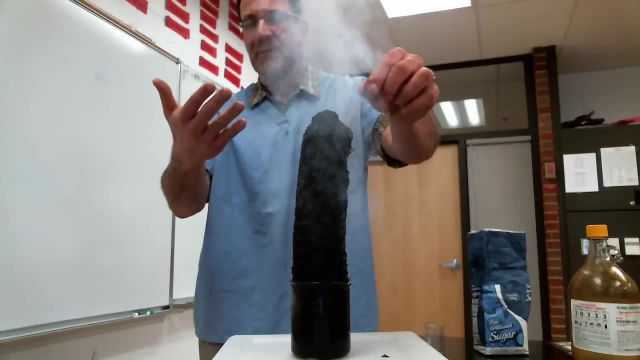 And the black stuff you see is carbon. The steam you see is mostly water. Of course it's a little bit of sulfuric acid in there, so you don't want to breathe it, But sugar will decompose into carbon. That's the black that you see. 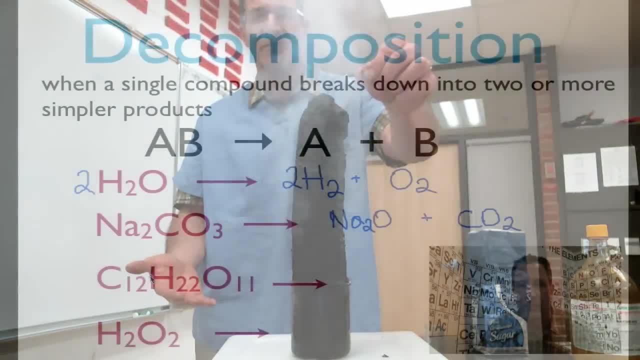 And then most of the steam you see is water, because sugar decomposed into carbon. Okay, That's always a kind of attention getter. You get that white sugar being broken down, being decomposed into carbon. That's the first step, And then the second step is also a kind of attention getter. 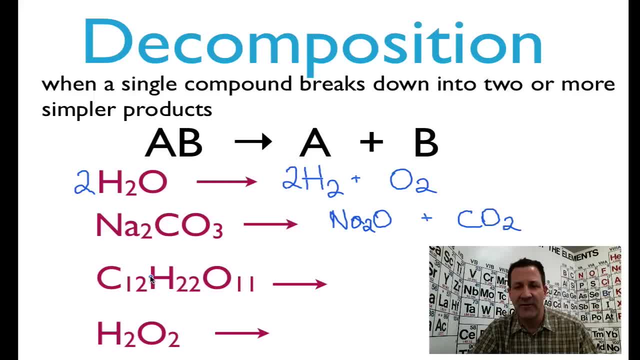 You get that white sugar being broken down, being decomposed into carbon and water. The carbon is the black stuff that comes out, a beaker like that, And then there's water in there also. It's kind of an exothermic reaction because it gets kind of hot or it is. 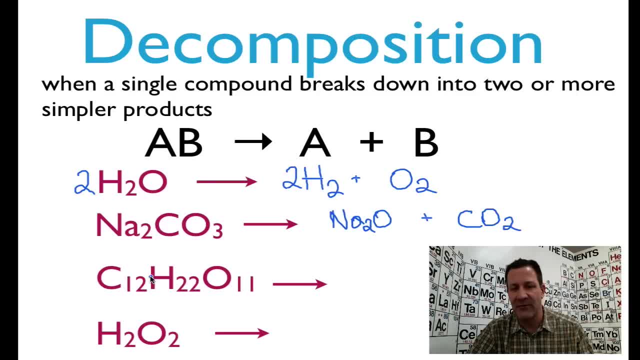 an exothermic reaction. It gets hot And there's some steam that comes from that. So let's go through and balance that. Let's see, We know that we're going to have carbon. We saw the carbon is just C, And then we know the other product is going to be water, So that's just H2O. 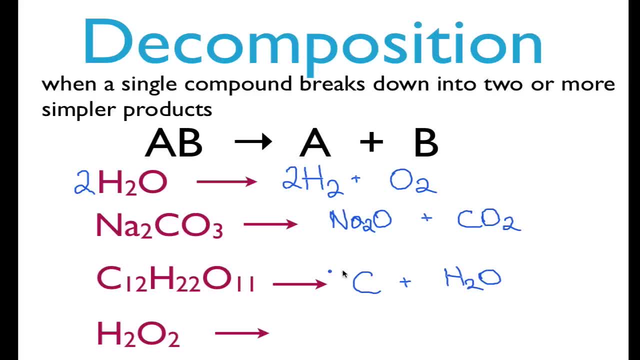 And we want to balance that. We have 12 carbons over here and we're going to have to put a 12 here, And in water there's a two to one ratio of hydrogen oxygen. You see, over here we have a two. 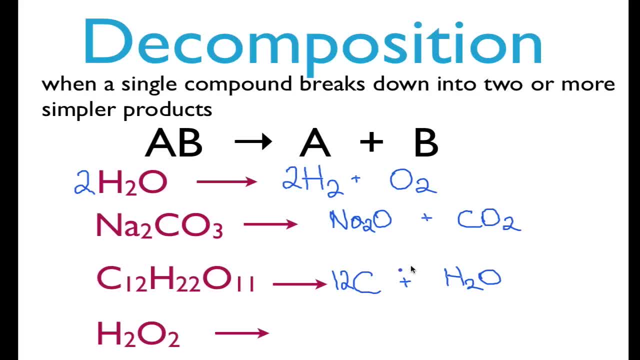 to one ratio of hydrogen oxygen in our sugar. So we know that we're just going to put an 11 right there, like that. Okay, I think that is balanced, just like that. All right. Now the last one we're going to do is hydrogen peroxide. We can decompose hydrogen peroxide And I'm going 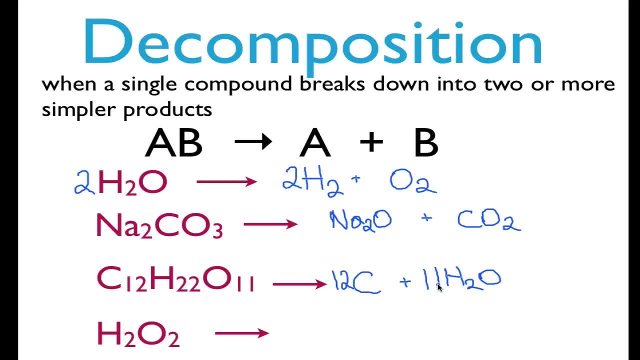 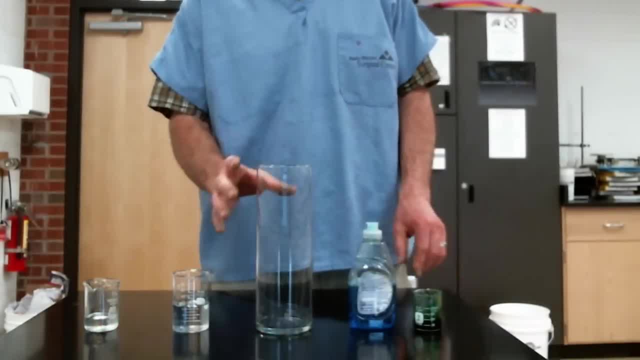 to show you this reaction too. This is a good one. This one is known as elephant toothpaste, So let's go and do that decomposition reaction right now, And then we'll come back. Now we're going to be doing the decomposition of hydrogen peroxide, So I have just here a 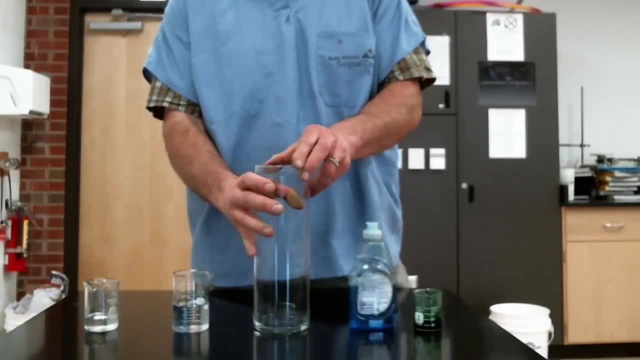 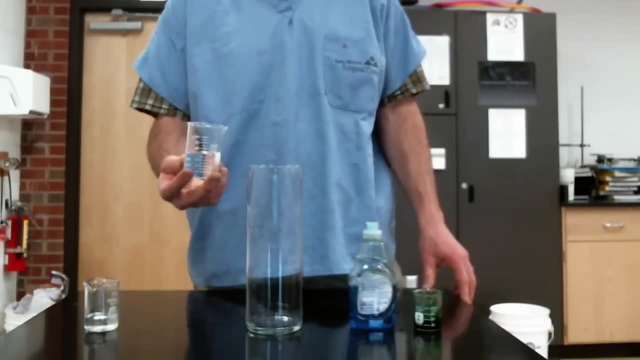 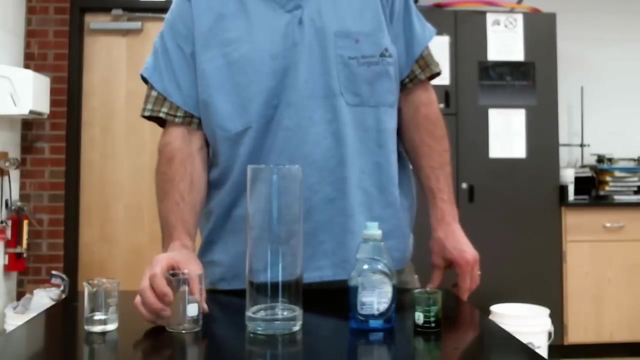 plain glass cylinder- I think this was a flower vase at one point- And to that I'm going to add about 80 milliliters of concentrated hydrogen peroxide. I think it's 35% hydrogen peroxide. All right, Now to that I'm going to be adding some food coloring. The food coloring is just for. 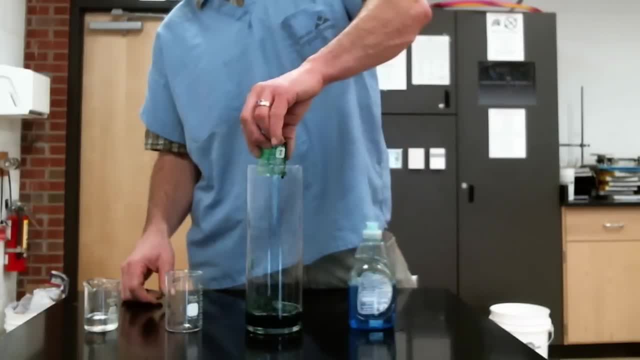 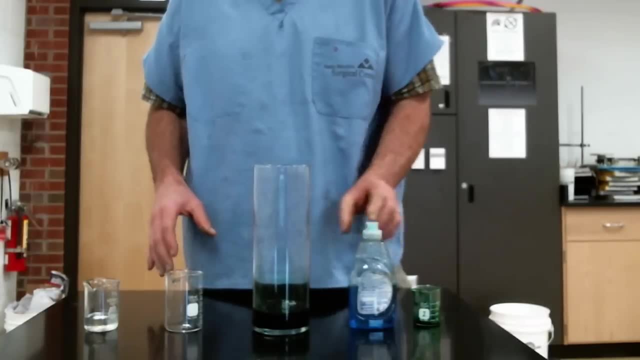 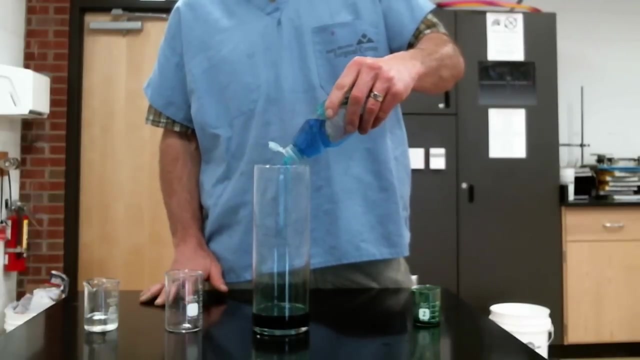 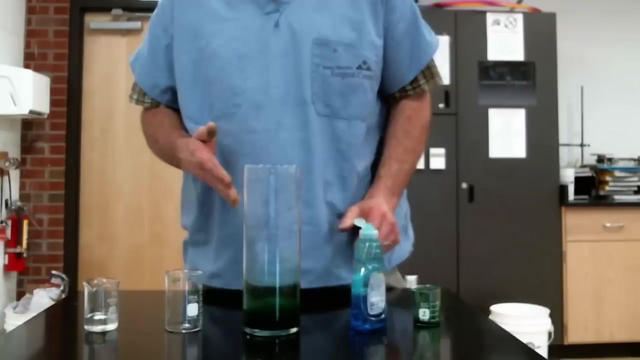 effect. You see, I have here green food coloring. Mix that up, And then to that also I'm going to be adding some plain dishwashing soap. This is just so we'll get some bubbles out of it. The food coloring and the soap are not part of the reaction. Okay, So I'm going to mix that up like that. Now we have 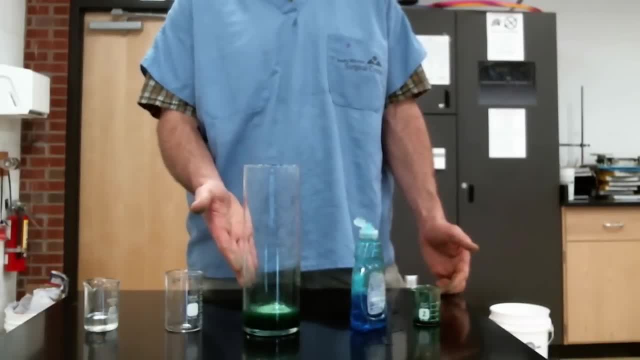 hydrogen peroxide in here And eventually, if we stand here and wait long enough, all the hydrogen peroxide will decompose And then we're going to add some hydrogen peroxide And then we're going to mix that up. We're going to add this one. Okay, Now we're going to add more hydrogen peroxide. 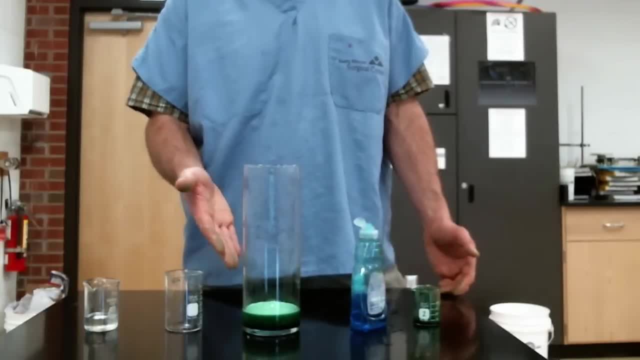 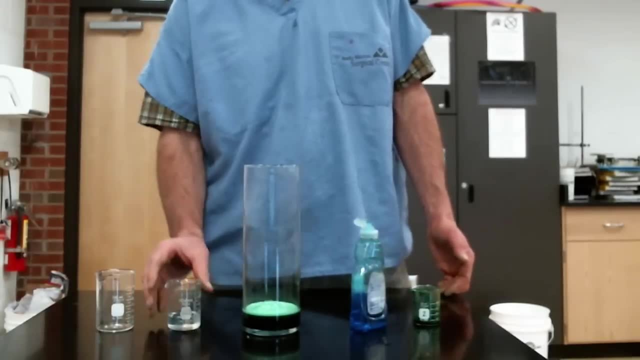 It will decompose into water and oxygen gas. But we want to make it look a little more interesting. We want to happened more quickly. So we're going to use a catalyst, And the catalyst that we're going to use is sodium iodide. So I have a solution here of sodium iodide And to the hydrogen.